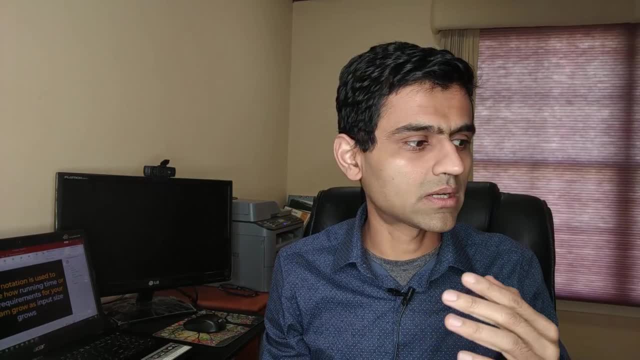 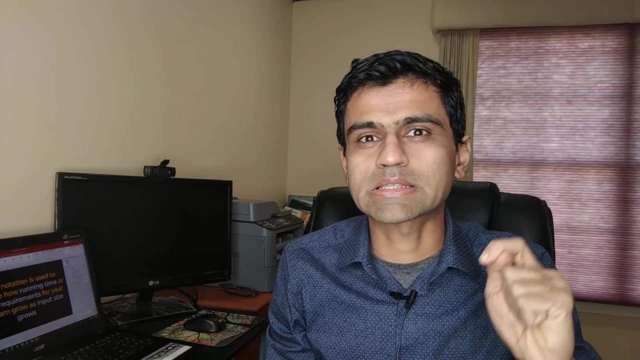 The first thing that you have to make yourself familiar with when you start learning data structures and algorithm is big O notation. I have not seen any programming interview where they don't ask about big O notation, data structures and algorithm. In this video, I'm going to tell you. 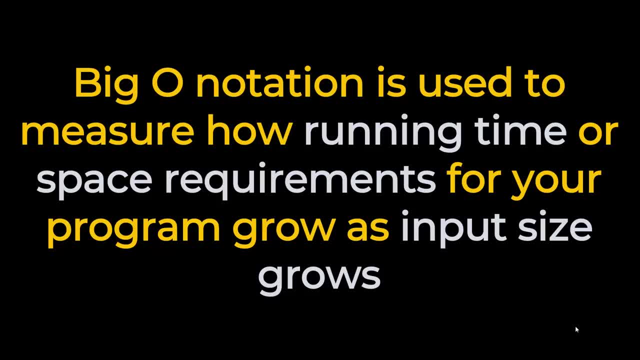 what is big O notation? by using few simple examples. Big O notation is used to measure how running time or space requirements for your program grows as the input size grows. In this video we are only talking about running time. Let's say you have this function, foo, which takes 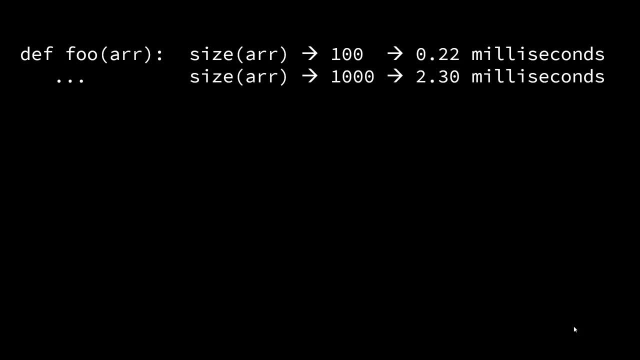 an array or a list as an input and it does some processing and it returns some output. When the size of array is 100, it runs in 0.22 millisecond. When it's 1000, it takes 2.3. 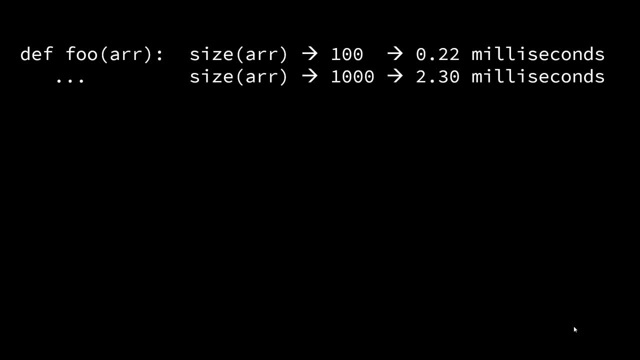 milliseconds. So as the size grows, the time also grows, And let's say: this is the graph of size versus time. You can clearly see that it's a linear function. The time that it takes to run this program is linearly proportional to the array size, and any linear function can be. 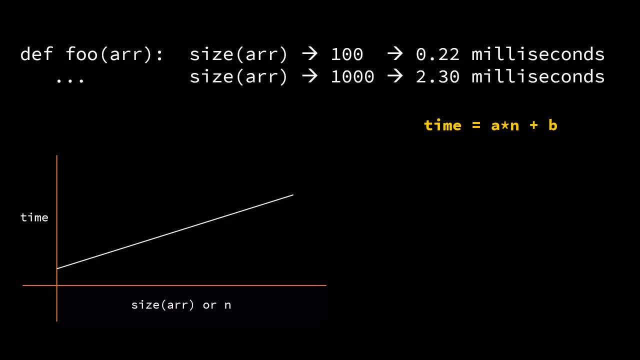 represented as a cross n plus b. Now the reason we are using a mathematical function here to measure the time requirement is because, depending upon the computer, this time might be different. I have a fast computer, So let's say it's 2.3 millisecond, But if you're a slow computer it might even take. 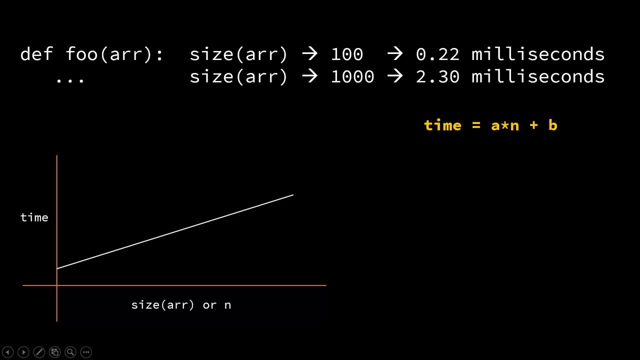 five milliseconds. So measuring time of the program in absolute terms is not useful. It has to be mathematically represented And that mathematical representation is big O. Here we are not going to say the time is a big O of a cross n plus b. 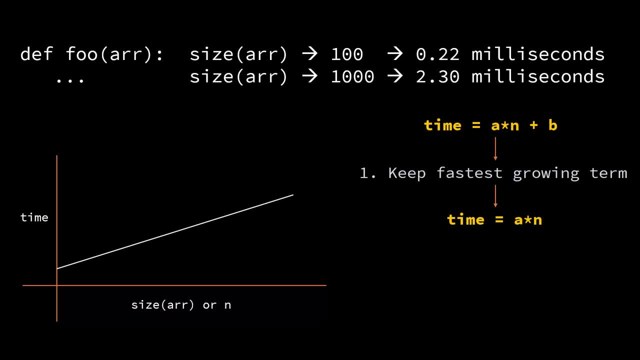 But we are going to apply some rules. So the first rule is we are only going to keep the fasted growing term. The b here is constant. So as the size of n grows, let's say n is 100. And a is 2, right, So it will be 200.. But when n becomes million, when you multiply by 2, it becomes. 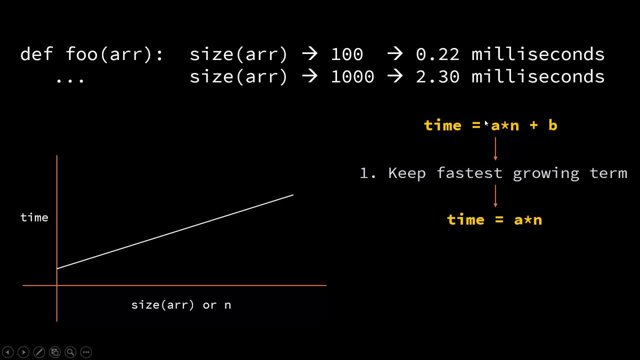 like 2 million, versus b remains constant. So the fasted growing term is a cross n. So we only keep that. The second rule is we drop any constants. So constant is a and we drop it, So what is left is n. And now we say the big O time complexity for this program is order of n. This is the example. 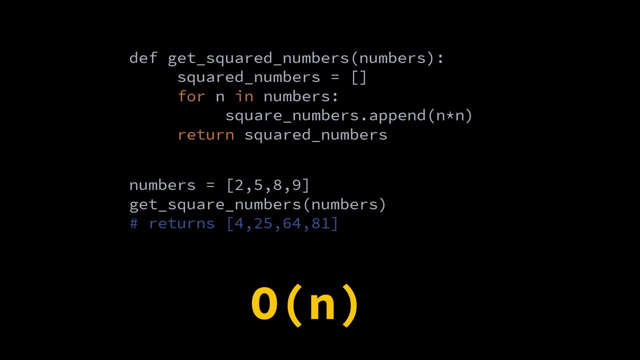 of a program whose time complexity is order of n. Let's say you are squaring the numbers by taking an input list. So this is the Python program. And now let me clarify. this big O notation is used for all programming languages. It is not specific to Python. I'm just using Python as an example here. 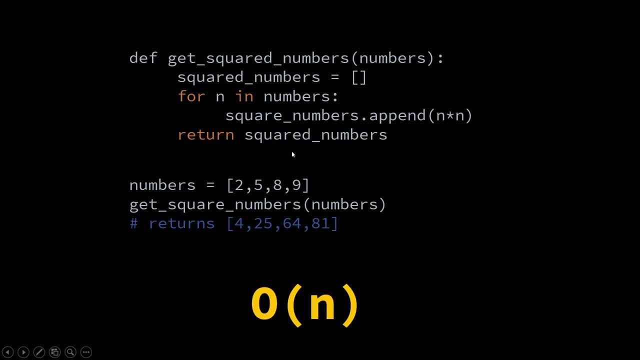 In this example you are running n iterations. So right now my array size is four, So it did four iterations. But let's say, if my array size is four million, it's going to do four million iterations And, as you know, the time that it 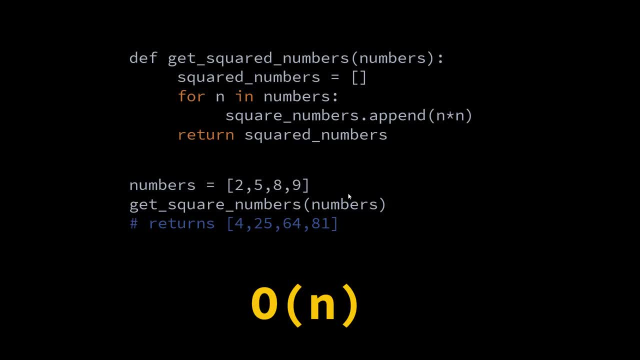 takes to execute the program is equally proportional to number of computation it is doing Here. if the size is four million, it is going to do four million computation in this four loop. Hence the time will grow linearly. Therefore the time complexity for this program is order of n. 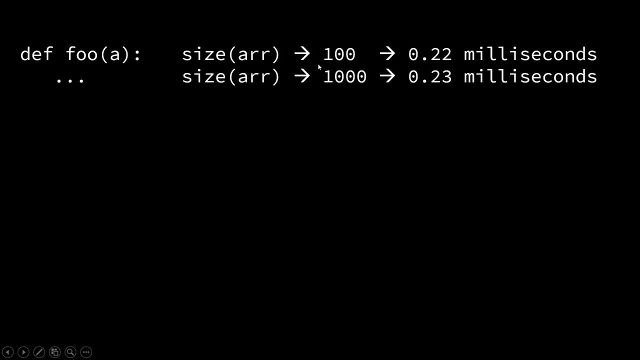 This is another example where when you increase the size of an input, the time is almost constant. It changes, but only a little bit. So you see like 0.22 and 0.23 millisecond. So the graphical representation of the time as the input grows. 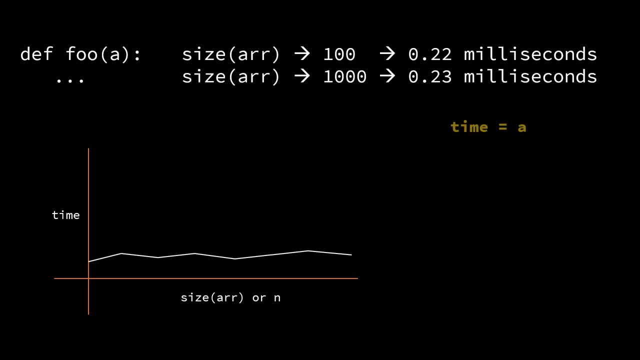 could be this: And it's a constant function. And constant function can be represented by time equal to a, where a is the constant. And when you apply those two rules, what you get is order of one complexity, Because the way you can look at a is a. 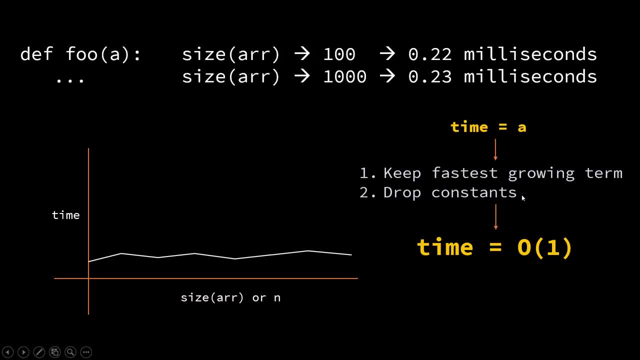 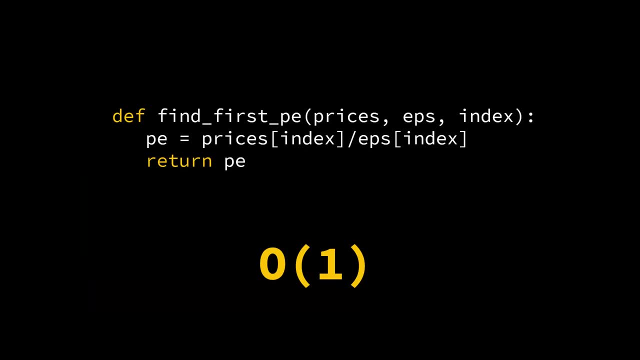 cross one And then by second rule, you can drop that constant, which is a, And what you get is order of one. This is the example of a function whose complexity is order of one. Let's say you are trying to find the P of the first stock in your list. So here I'm, getting the stock price In a. 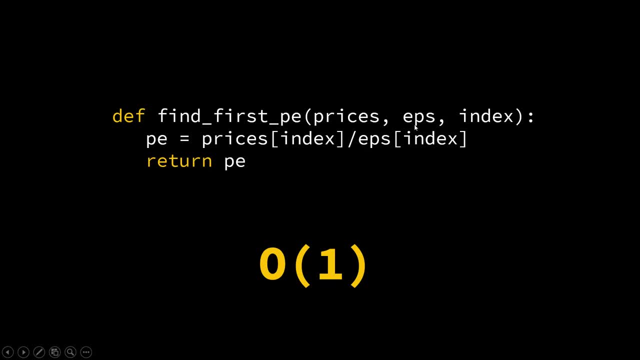 list. I'm getting EPS of different stocks in the list, So these two lists have price and EPS for different stocks. There could be ten stocks or a million stock, But when you supply an index it is going to do a constant operation, So it doesn't matter what is the size of price or 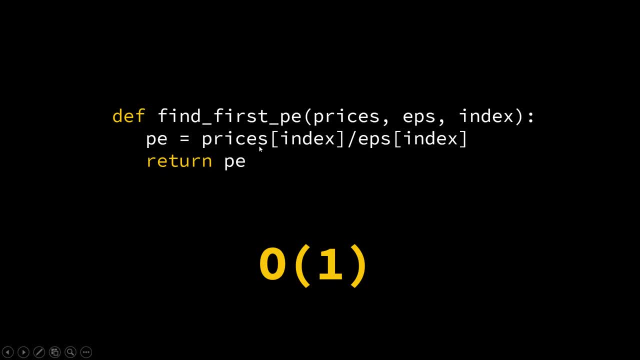 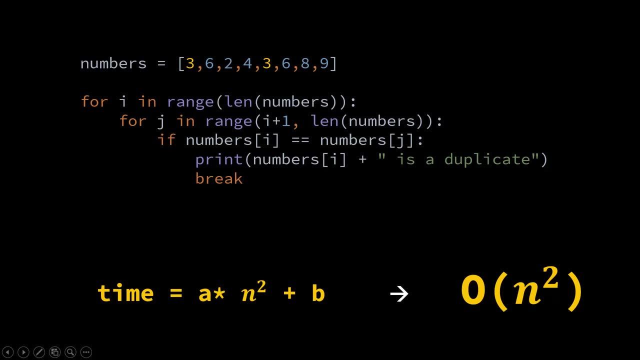 EPS, It could be ten, It could be a million. The time execution is going to remain constant, Hence the big O. complexity of this program is order of one. This is another program where you are trying to find a duplicate from your list. Here we are running two for loops. 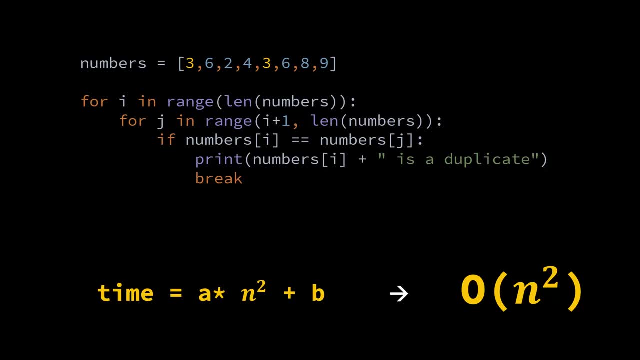 And you are comparing the numbers in two for loops and trying to find a duplicate. You might be aware about this program. The linear equation for the timing of this function, as the list grows, is a cross n square plus b. This is the standard linear equation And here, when you keep only the 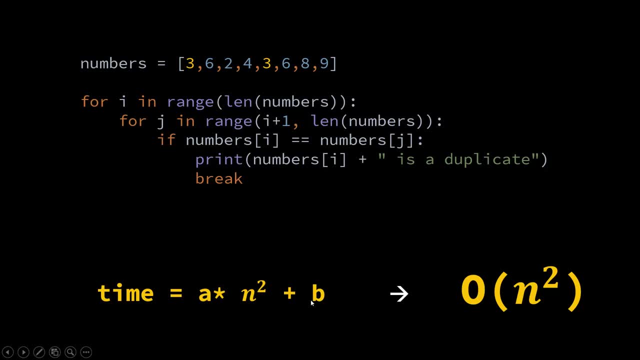 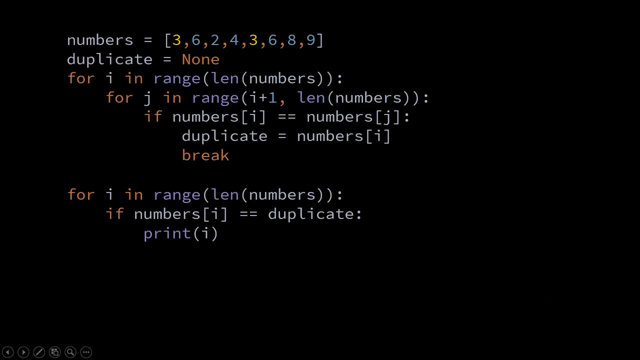 fastest growing term, which is a n square, and drop the constant, such as b and a, you will get order of n square. Here is another example where, in this program, the first block of code is doing n square iteration, The second block is doing 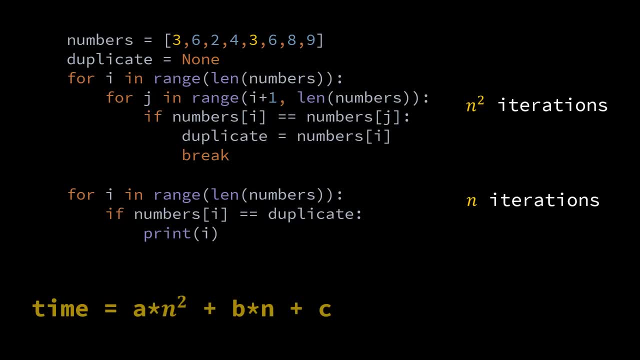 an iteration. So to represent the time you can use this equation: a? n square plus b? n plus c. But in this equation again apply those two rules: Keep the fastest growing term, which is a? n square, Drop b? n, b n plus c, and then also drop the constant, which is 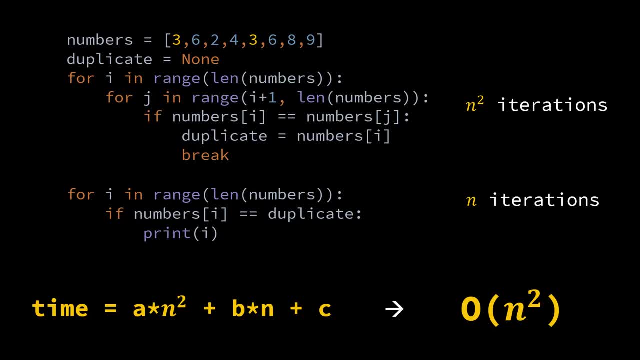 a and then you get order of n square complexity. So sometimes people say the complexity of this program is order of n square plus n, But no, it is order of n? square. And I will explain you why you apply those two rules. Why do you keep only the fastest growing term? 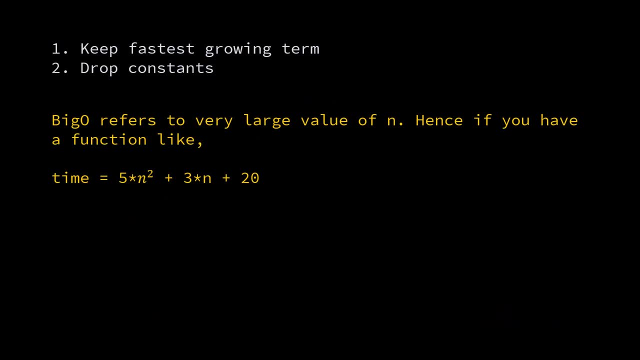 So let's understand that the reasoning behind these two rules. Let's say you have a function which is something like this: phi, n square plus three, n plus 20.. Now big O is a very rough ballpark estimate. It refers to the value of n, which is very large. 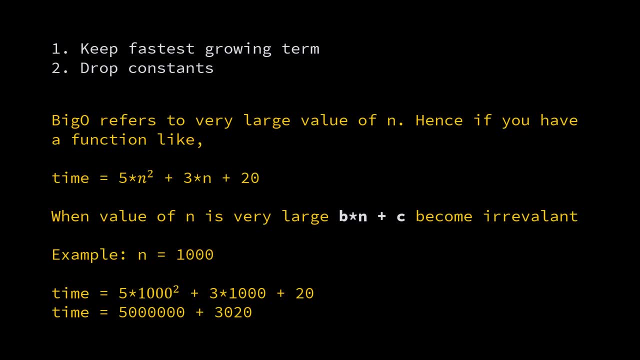 I'm not going for any large value here, But let's say even if n value is 1000.. In that case, in this equation, the first term will contribute the most, it will be 5 million, whereas the second and third term will come around 3020.. Okay so, 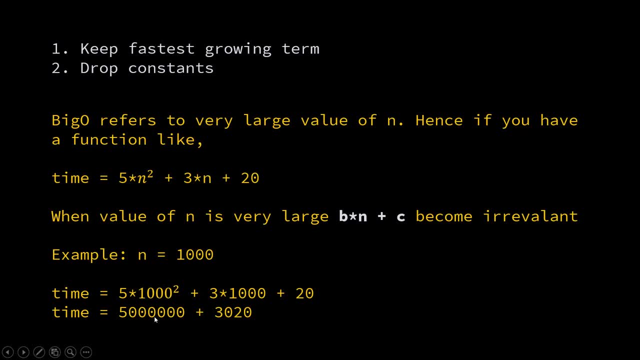 3020 is very minor against 5 million value. hence it can be dropped. Big O is a simplistic method of saying: this is how much my program is going to take. Hence it makes sense that you only keep the fastest growing term and drop everything else. Until now, whatever we saw was for running time. 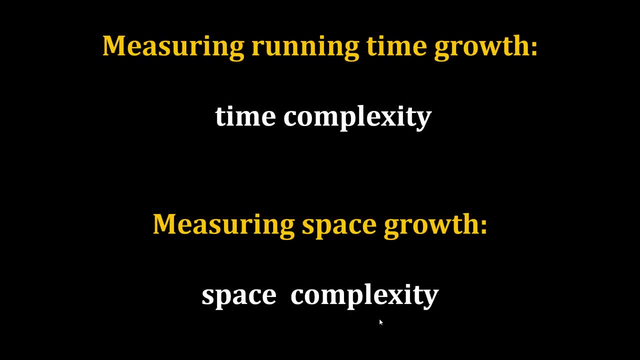 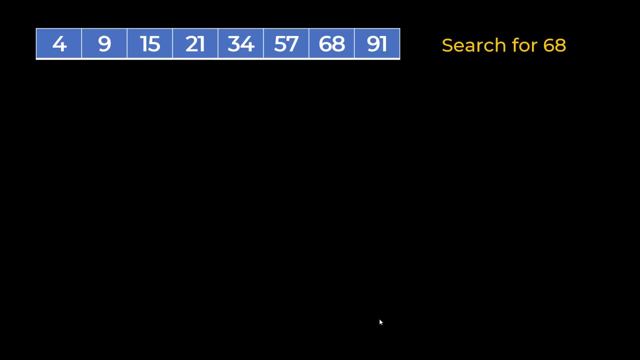 growth. it is called time club complexity, But the same can be used to measure the space growth. And the next one is called space complexity. Let's look at one more example of binary search. When you have a sorted list of numbers if you want to search for a specific number. 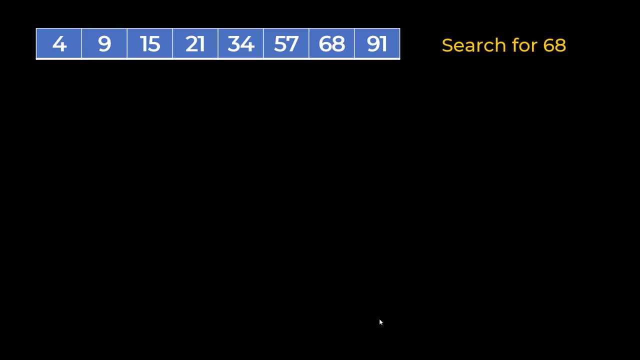 how do you do that In this example? I have eight numbers. I want to search for 68.. Simple method is you go through all the numbers one by one and compare again 68 and find the index. This has order of n complexity. This is a very simple example, So this program will run fast. but 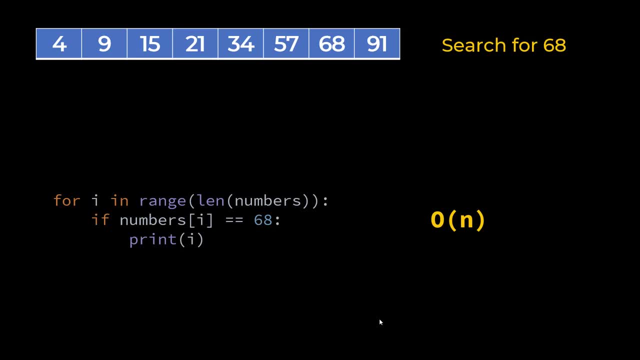 let's say you have billion numbers in your list And you want to find out the index of a specific number. you don't want to do billion iteration because it might be very time consuming. There is a better way, which is binary search. In this what you do is you first find the middle element. 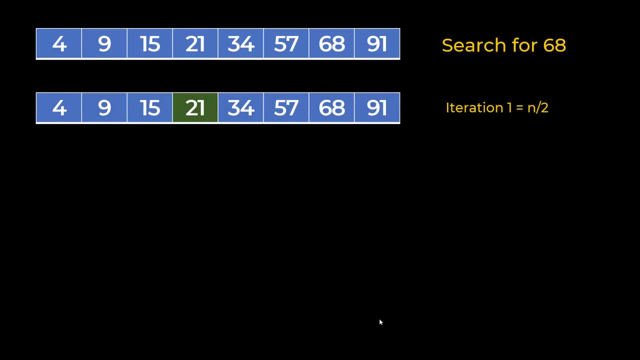 which is 21,. you compare it against 68, you find out that 21 is less than 68. Hence you now discard the array on the left hand side, So number four to 21,. you discard it And now what you have is 34 to 91. In that array also. 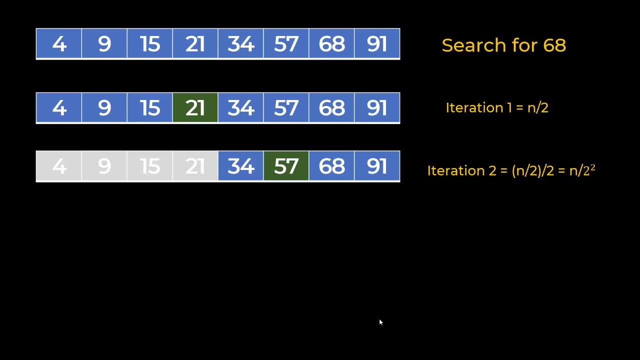 you find the middle element. So you basically, in each iteration you are dividing the array by two. Here the middle element is 57. Again, compare it with 68.. 57 is less than 68. Hence you discard the left hand side array, which is 34 and 57. You now have only 68 and 91 in your search space. 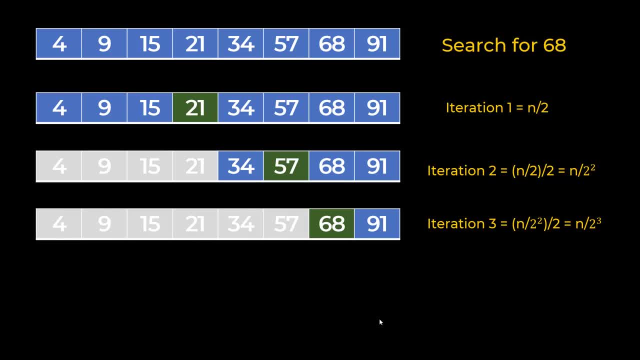 Again, you divide it by two, you take the middle element, which is 68. And 68 is the element you were looking for. So you found your answer in three iteration. if we had done an iteration, which is a previous approach, we would have taken seven iteration, because the element is: 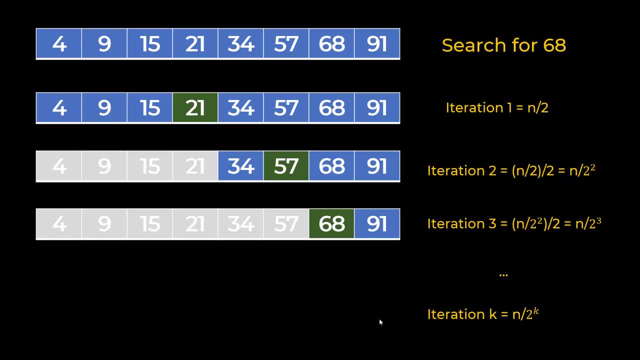 the seventh number. Okay. so this is better if you have big array And if you are doing like key iteration. equation on the right hand side shows that for iteration key you have to do and divide by two, raised to k operation for key iteration. Now let's convert this into big O. 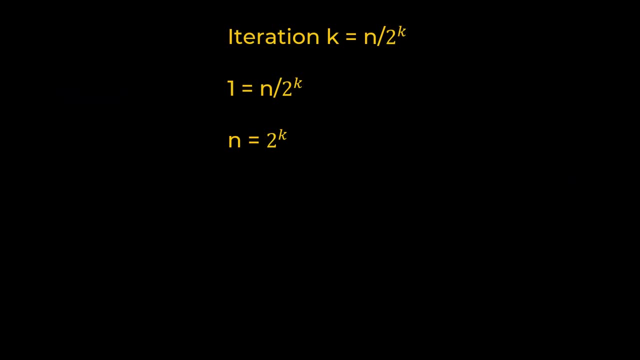 So we have to do n divided by two, raised to k iterations to get the array size to one one, because that is our worst case estimate. Okay, you might find your answer in less a first iteration itself if the element you're looking for is exactly in the middle. But big O notation is used generally to measure performance in worst. 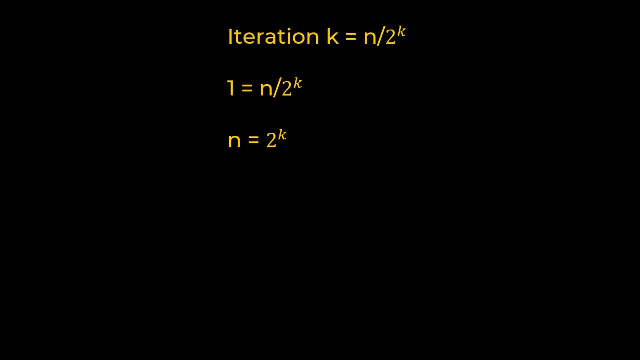 case scenario. So we always talk about worst case scenario when we are thinking about big O notation. here are to reduce the array size to one. you have to do n divided by two raised to k iteration And that you can represent in this equation. So here, two raised to k you can take. 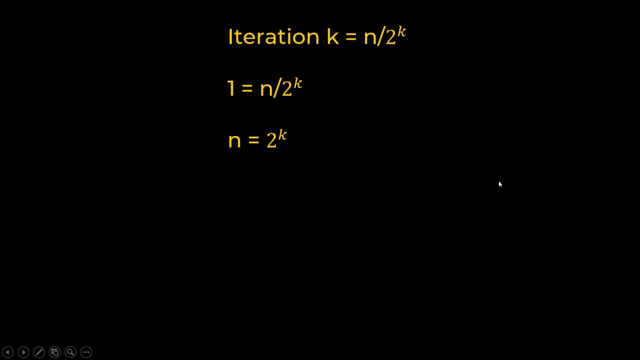 here and it becomes: n is equal to two raised to k. After that you can apply log to the base two on both sides of your equation. you get this Now. you know that this log, this right hand side equation, you can represent as k. 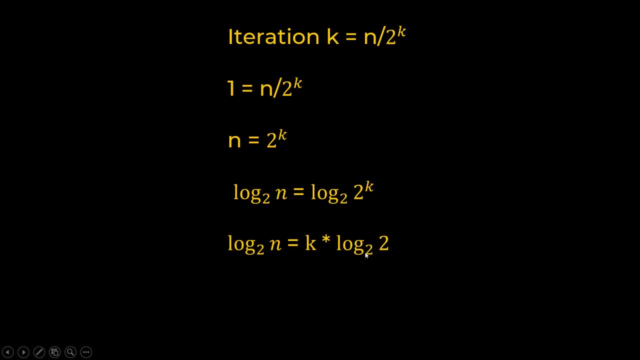 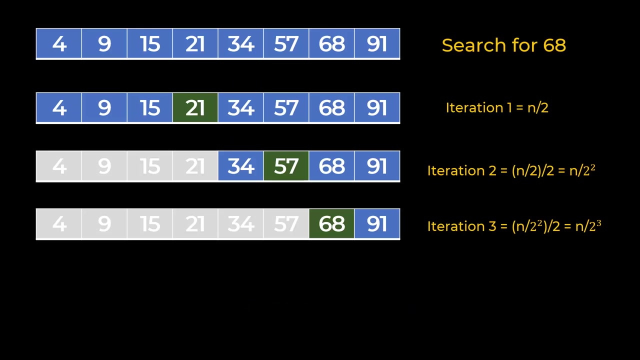 into log two, base two. now log n. base n is one, So this part becomes one. Hence my k, which is number of iteration. that I need is log n. Hence the complexity of binary search. is order of log n. Here I had eight elements, So for eight elements, 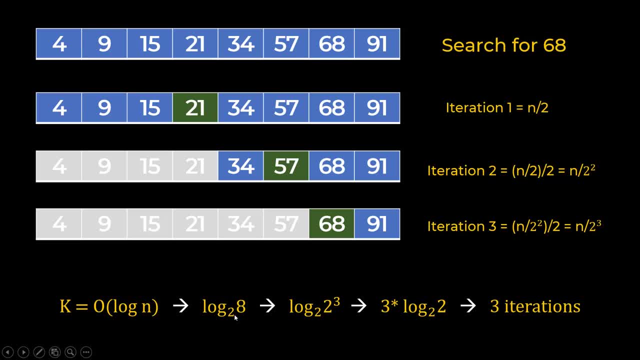 I can apply order of log n equation And it will be eight. you know it's two raised to three, three comes ahead and log two to the base, two becomes one. Hence you find the answer that this is three iteration. When you go to programming interview, often they will ask you a question. 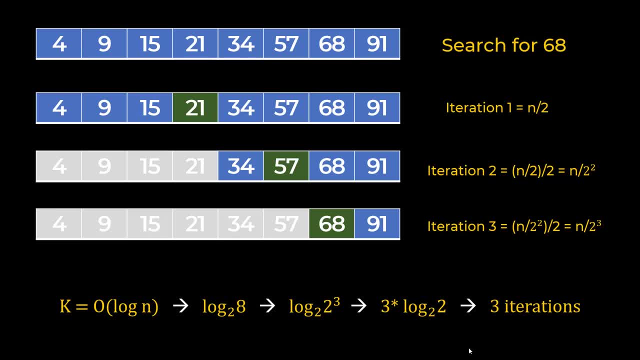 And let's say, for this binary search problem, let's say you did order of an iteration, which was our first primitive approach. the interviewer will ask you: can you do the same thing with a better performance? Or they can say: Oh, this.